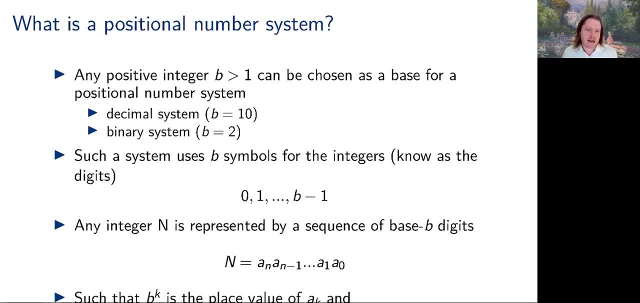 going to be kind of, they're going to have very similar characteristics. So what is a positional number system? So any positive integer that is greater than 1 can be chosen as a base for a positional number system. The decimal system uses a base of 10.. The binary system uses a base of 2.. 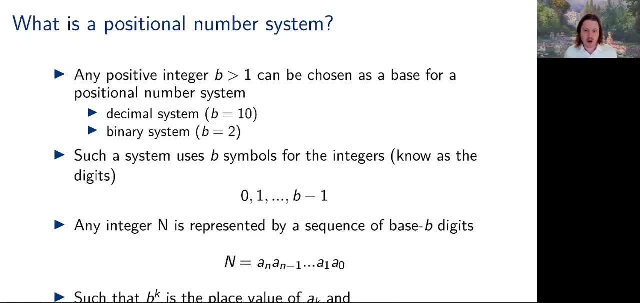 Such a system will then use b symbols for the integers, known as the digits. So you'd have 0, 1, all the way through b minus 1.. So the digits in the decimal system are going to be 0 through 9.. 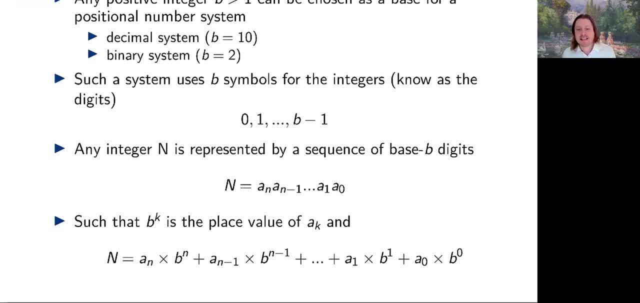 Now any integer in the decimal system is going to be 0 through 9.. So the digits in the decimal system can be represented by a sequence of those base b digits. For instance, in base 10, we might have seen something like 1,, 0,, 1,, 2, or 1,, 0, and 12.. This is simply a sequence of those. 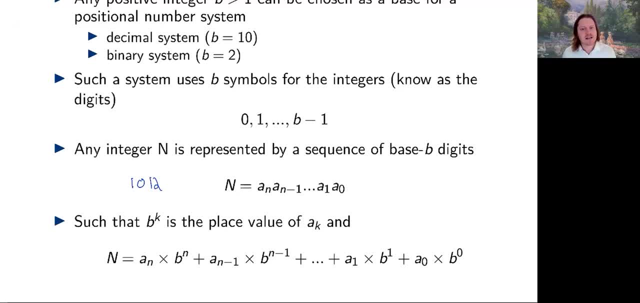 base b base, in this case base 10 digits 0 through 9. So we have one digit here- 2, another digit 1, another digit 0, another digit 1.. I mean, we could have had alternatively. 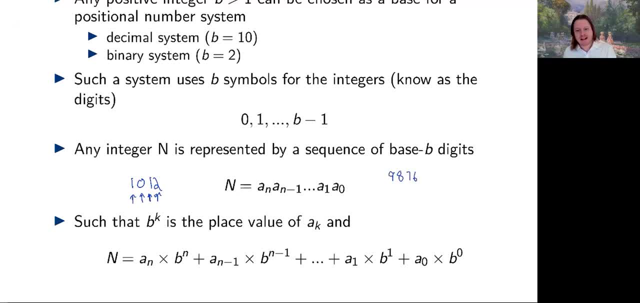 a sequence of like 8,, 9,, 7,, 6.. But again we can see here that an integer number, some integer number n, is simply going to be represented by a sequence of the digits in our positional number system And then kind of the key takeaway at this point is to realize that where a digit presents 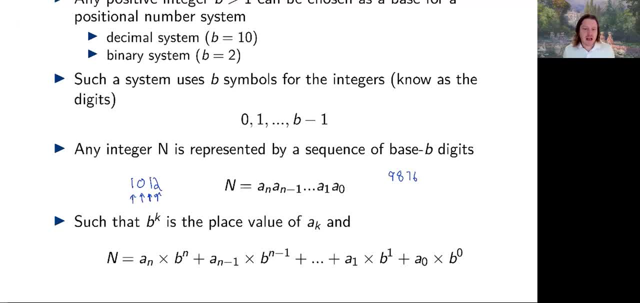 in the sequence is going to have an implication in terms of how much it is contributing to the overall number, or integer value, Since we can see here that that 6 is going to contribute simply 6 to the overall number. that 7,, based on its position, is going to contribute 70.. That 8,, based on its position, 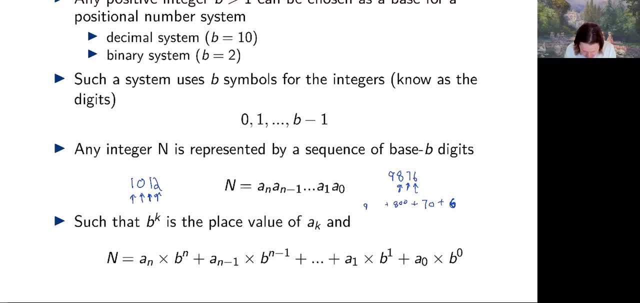 will contribute 800.. And then that 9,, based on its position, is going to contribute 9,000.. And when we add up all of these values, what we're going to get is 9,, 8,, 7, 6.. 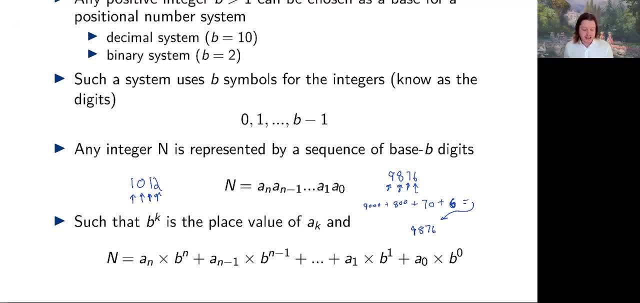 So we can see here that the digit at some position is going to be the place value of that position, And to find the number it's simply going through and adding up the digit multiplied by the place value of that position to come up at the actual integer value expressed. 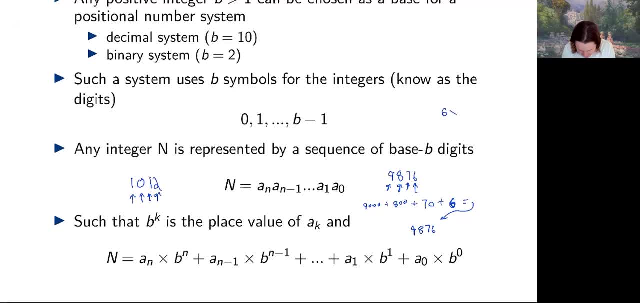 So here that would be 6 times 10 to the 0,, because we're at position, in this case, 0, from right to left, And that's going to evaluate to 6.. We're then adding 7 times 10 to the 1,, which is going to be 70,, plus 8 times 10 to the 2,. 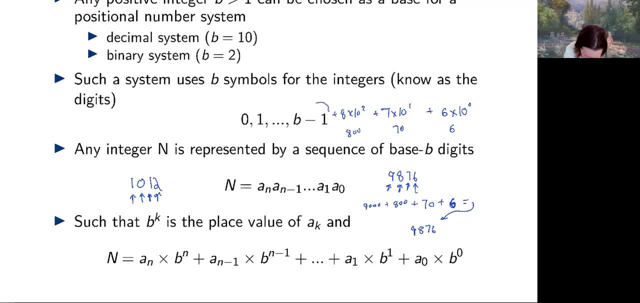 which will be 800, plus 9 times 10 to the 3,, which is going to be 9,000.. And adding these together again, we get that. We get that value: 9,, 8,, 7, 6.. 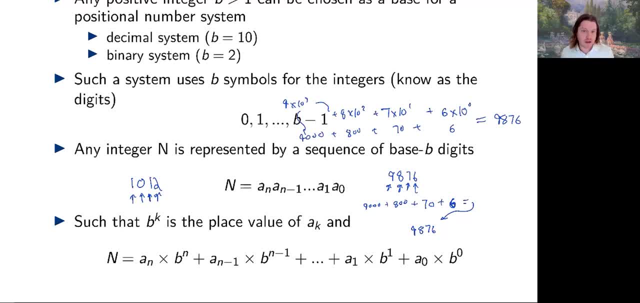 And the key to take away here is that, as you're moving from right to left and evaluating this sort of integer value- in our example here in base 2, we would go ahead and call- oops, I did not mean to erase. We would go ahead and say the value 6 occupies position 0,. 7 occupies position 1,, 8 occupies. 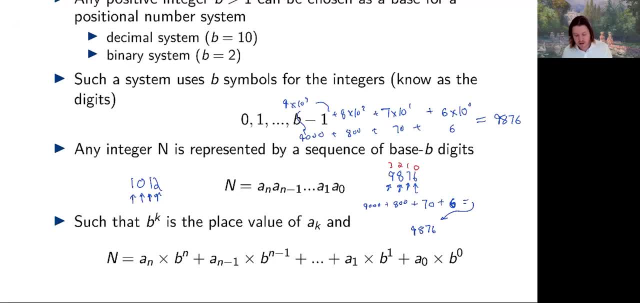 position 2, and 9 occupies position 3.. And that's where we got these values here, where n is going to be the position. So we can kind of think about any of these digits within this number: 9,, 8,, 7,, 6, contribution. 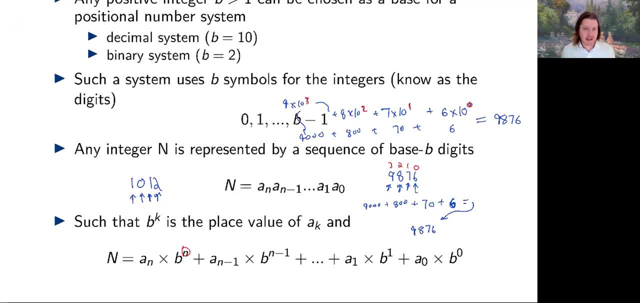 to the overall number, by looking at erasing it, rather to its position, to the base, to its position. So again, that's what we showed here. So, kind of moving on from this, Let's talk about the binary system. 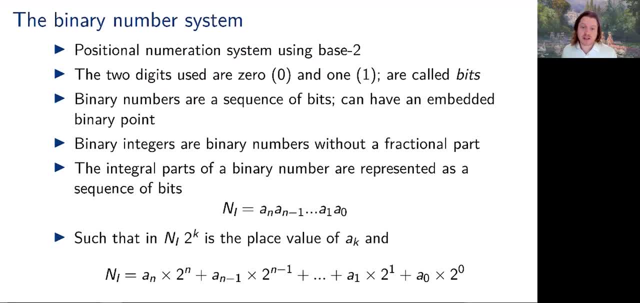 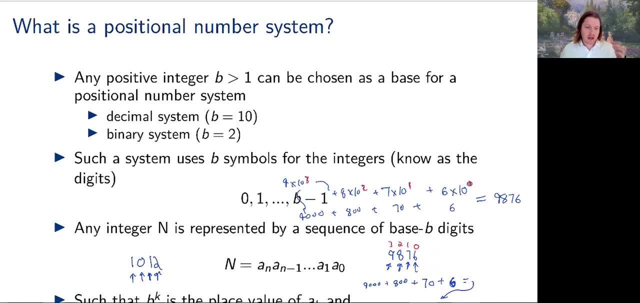 So this is simply going to be a positional numeration system using base 2, the two digits that are going to be used here- which, as we talked about up here, is simply the symbols that we can use- are going to be b minus 1.. 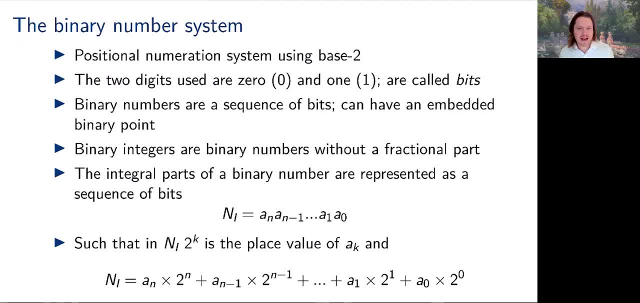 So in this case, if b is 2, we'll only have 0 and 1 as the digits in the binary system And we're going to call these bits. Binary numbers are going to be composed as a sequence of bits and they can have an embedded. 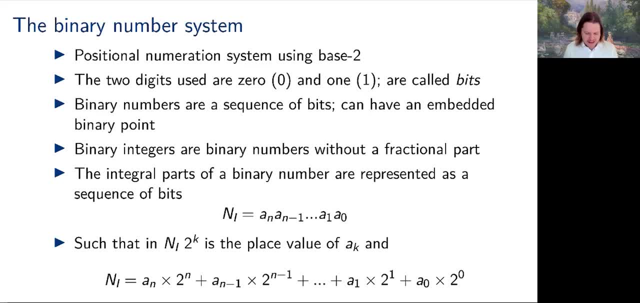 binary function. So this is going to be a binary point. just like in the base 10 system, you could have something like 3.14.. In binary, as a new number system, you could have something like 101.101.. 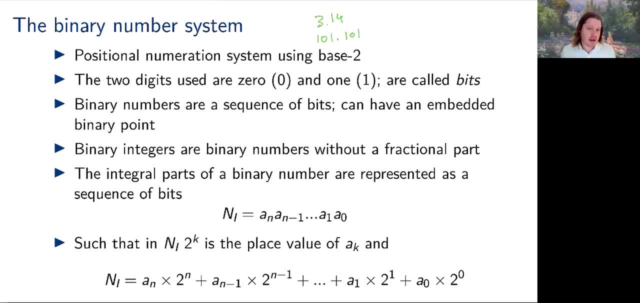 This is fine. But what we're going to see is that when we're talking about storing, say, binary numbers within the computer, well, we're not going to be able to just encode a dot somewhere in that number. So, due to this, I'm just going to kind of focus on binary integer values or binary numbers. 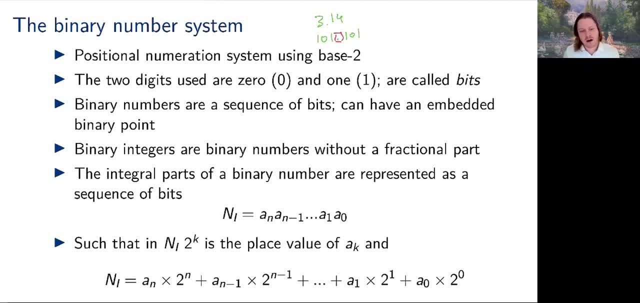 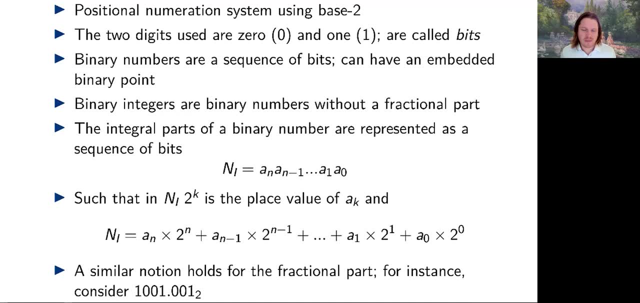 without the fraction part for the majority of this video and kind of continue through that until we hit the floating point values And we'll talk about how we can represent a floating point value as a binary integer. So without a fraction part and we'll see. it's kind of an interesting encoding scheme. 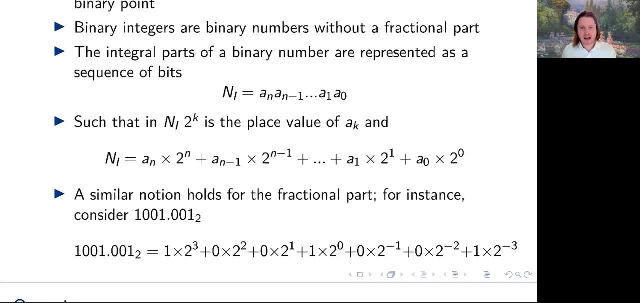 to do that, But most of what is presenting. But here is what we talked about for the base 10 system. Again, we just have less digits and we'll see here that as you move from right to left, the contribution of a particular binary digit in a binary number is going to be raised to. 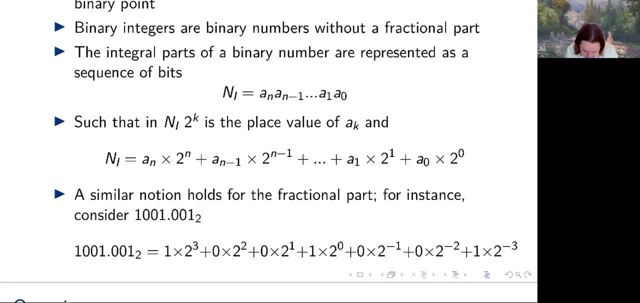 a power of two instead of 10.. So, if we had the binary number 101, and we wanted to know what this encoded in decimal. well, remembering back to our placeholders, and I'll use some lime green here, that's position one or zero, excuse me. this is position one. this is position two. 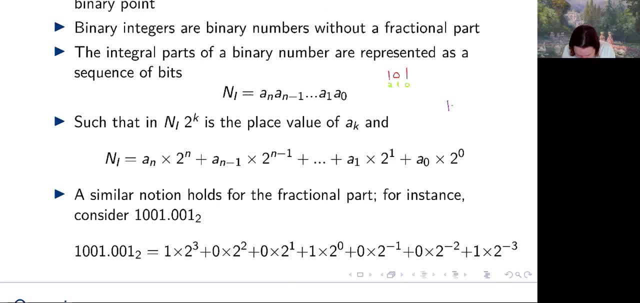 So, to go ahead and calculate this out, we would have one times the base raised to the position, which is zero plus zero times the base raised to the position, plus one times the base raised to the position. and if we go ahead and add this up, what we'll see is: 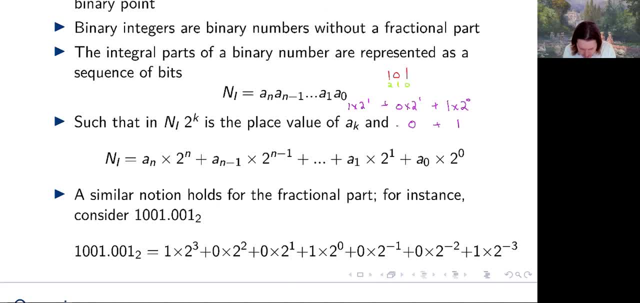 we're going to have one plus zero, Okay plus four, and that's going to add to five. So 101 is going to be equivalent, is going to be the base two equivalent of five in the decimal system. So we can see here that a lot of what we've talked